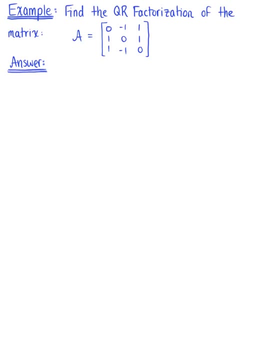 Find the QR factorization of the given matrix A, where matrix A is this beautiful 3x3 matrix. So let's keep in mind here that the goal is to rewrite this matrix A into the product of matrix Q and matrix R, where matrix Q is a 3x3 matrix with orthonormal columns and matrix R is an invertible upper triangular matrix. 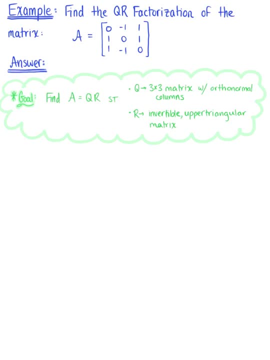 Now, hopefully this matrix looks familiar. We can recall that in a previous example we actually found an orthogonal basis for the column space of this matrix using the Gram-Schmidt process. So we can actually use this orthogonal basis for the column space of matrix A to find matrix Q. 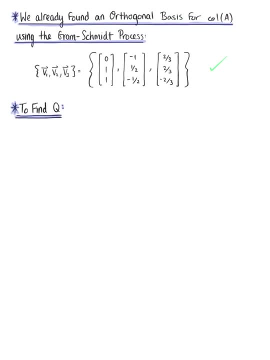 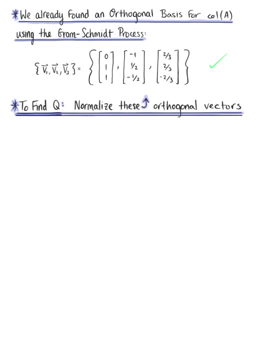 Since this is already an orthogonal basis to find matrix Q, all we need to do is normalize these orthogonal vectors. So here we go. We've got our first vector, vector Q sub 1, and to attain vector Q sub 1,, we are normalizing vector V sub 1.. 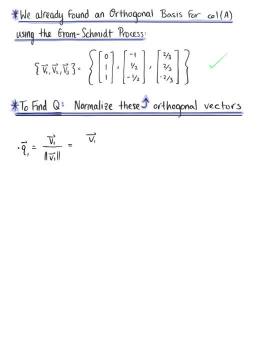 So we have vector V sub 1 divided by the magnitude of vector V sub 1, which is the square root of 1 plus 1.. So this leaves us with the scalar multiple 1 by the square root of 2 multiplied by the vector 1,. 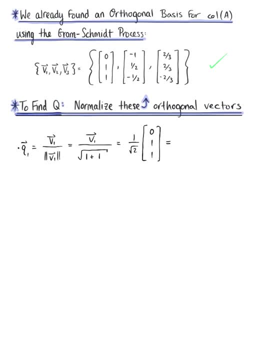 which is the vector with components 0,, 1,, 1, and distributing this scalar through, we have the vector with components 0, 1 by the square root of 2,, 1 by the square root of 2.. Beautiful. 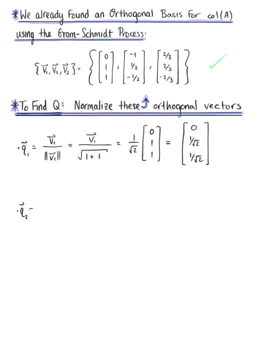 So now we need to find vector Q sub 2.. So to find vector Q sub 2, we are going to normalize vector V sub 2.. So we have vector V sub 2 divided by the length of vector V sub 2.. 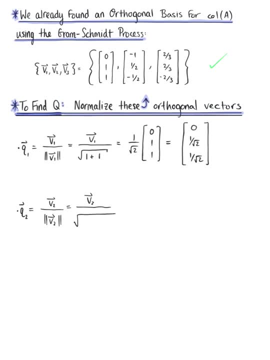 So we have vector V sub 2 divided by the length of vector V sub 2.. So we have vector V sub 2 divided by the length of vector V sub 2.. So this is the square root of 1 plus 1 fourth plus 1 fourth. 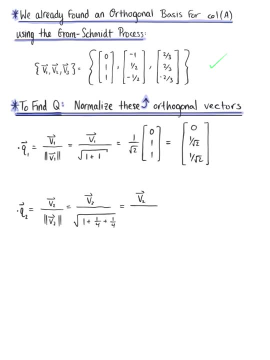 which is equal to vector V sub 2 divided by the square root of 3 halves. So simplifying this, we can rewrite this as the square root of 2 by the square root of 3.. Multiply by vector V sub 2, which is the vector with components: negative 1, 1 half. negative 1 half. 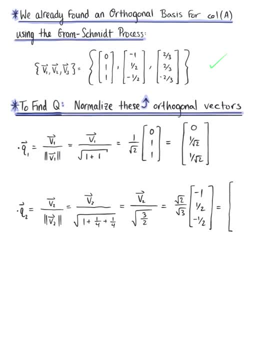 And distributing this scalar multiple through, we are left with the vector with components negative: square root of 2 by 3, square root of 2 divided by 2 times the square root of 3, and then minus the square root of 2 divided by 2 times the square root of 3.. 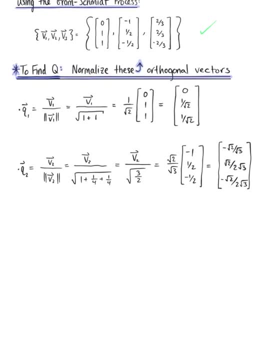 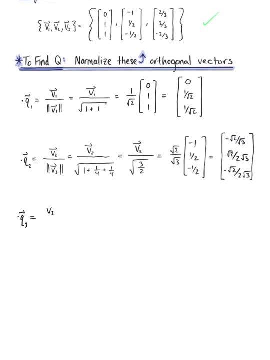 And last but certainly not least, we need to find vector Q sub 3.. And we find vector Q sub 3 divided by 2 times the square root of 3.. And we find vector Q sub 3 by normalizing vector V sub 3.. 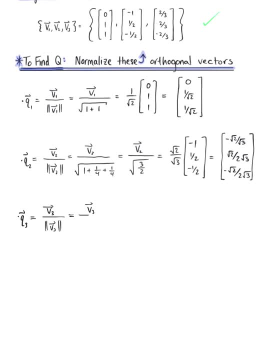 So we have the given vector V sub 3 divided by its length, which is the square root of 4 ninths plus 4 ninths plus 4 ninths. So this simplifies to vector V sub 3 divided by the square root of 12 ninths. 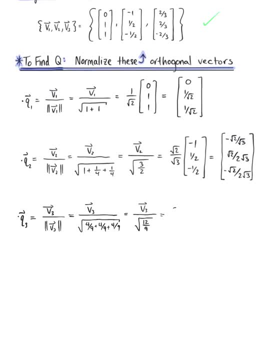 which we can further simplify To being 3 divided by 2 times the square root of 3, multiplied by the vector V sub 3, with the components 2 thirds, 2 thirds, negative 2 thirds, And distributing that scalar multiple through, we are left with the vector with components. 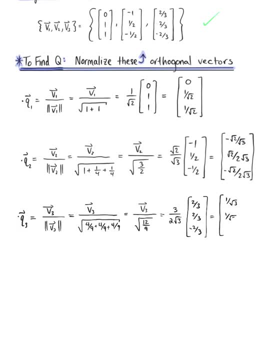 1 by the square root of 3,, 1 by the square root of 3, minus 1 by the square root of 3.. So, therefore, matrix Q is the 3 by 3 matrix, with column vectors Q sub 1,, Q sub 2, and Q sub 3.. 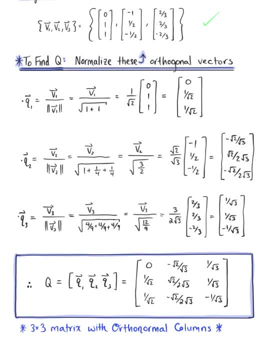 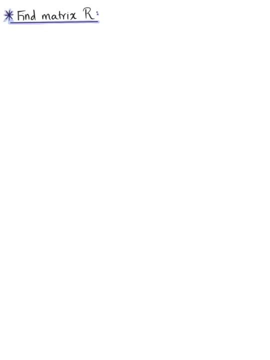 So these are orthonormal column vectors. They are orthogonal and unit vectors. So now that we have this matrix Q, we are ready to find matrix R. So how are we going to find this invertible vector? How are we going to find this invertible upper triangular matrix R? 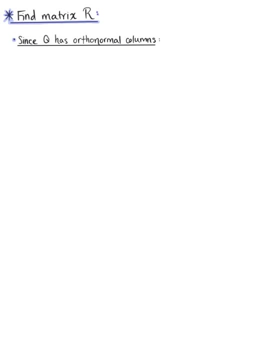 Well, using the fact that matrix Q has orthonormal columns, we know that the product of the transpose of matrix Q with matrix Q is equal to the identity matrix. So, with this identity in mind, let's left-hand multiply the QR factorization equation. 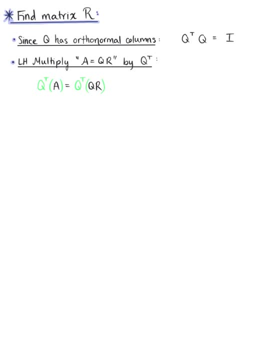 by the transpose of matrix Q. Now, simplifying the right-hand side, we can reduce this down to matrix R. So in other words, matrix R is equal to the transpose of matrix Q multiplied by matrix A. So that's how we will find matrix R. We need to compute the transpose of Q times matrix A. 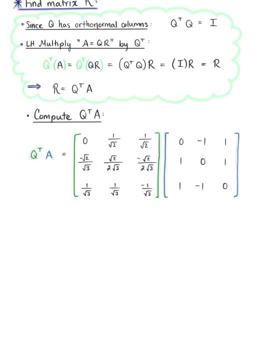 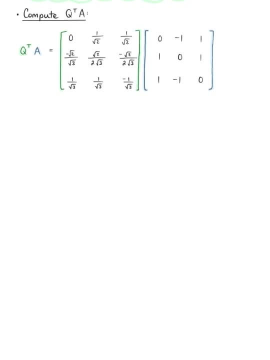 And giving ourselves plenty of room. we are going to compute this matrix matrix using the row-column rule, So this is going to be equal to: we have the first row times, the first column, which is 0 plus 1 by the square root of 2 plus 1 by the square root of 2.. 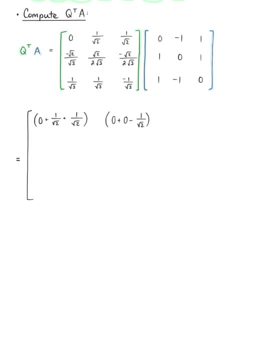 First row times the second column 0 plus 0 minus 1 by the square root of 2.. First row by the third column gives us 0 plus 1 by the square root of 2 plus 0.. Second row by the first column leaves us with 0 plus the square root of 2 by 2 times the. 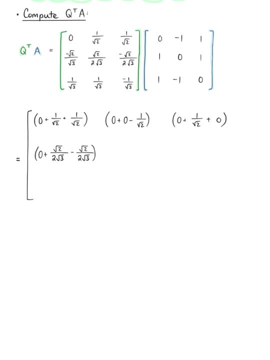 square root of 3 minus the square root of 2 by 2 times the square root of 3.. Second row times. the second column leaves us with the square root of 2 by the square root of 3 plus 0, plus the square root of 2 by 2 times the square root of 3.. 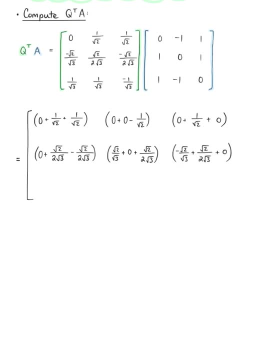 Second row times. the third column leaves us with minus square root of 2 by the square root of 3 plus the square root of 2 by 2 times the square root of 3.. Second row times: the third column leaves us with minus square root of 2 by the square root of 3 plus the square root of 2 by 2 times the square root of 3..